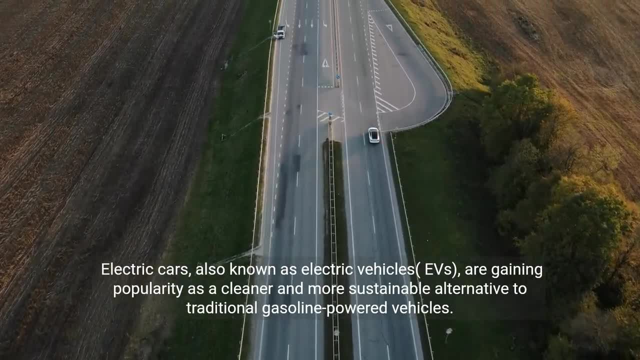 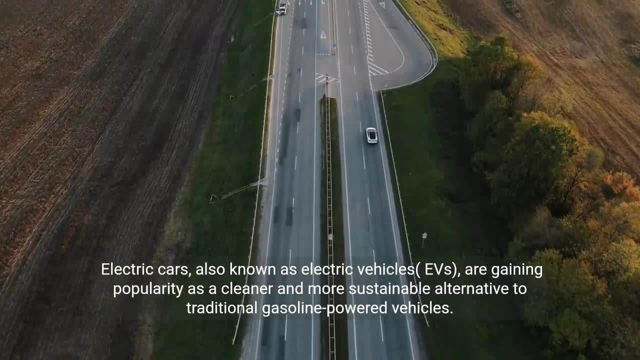 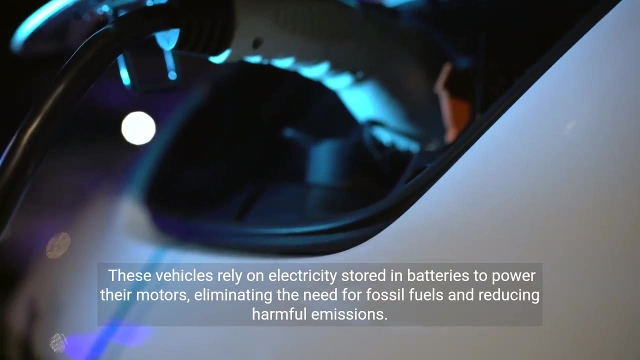 Electric cars, also known as electric vehicles. EVs, are gaining popularity as a cleaner and more sustainable alternative to traditional gasoline-powered vehicles. These vehicles rely on electricity stored in batteries to power their motors, eliminating the need for fossil fuels and reducing harmful emissions. Understanding how electric cars work involves delving into 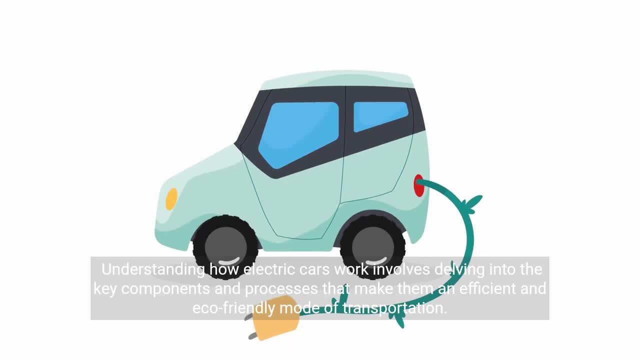 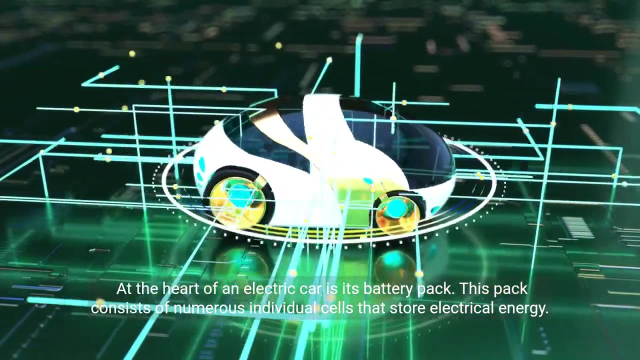 the key components and processes that make them an efficient and eco-friendly mode of transportation. At the heart of an electric car is its battery pack. This pack consists of numerous individual cells that store electrical energy. These cells, typically lithium-ion batteries, are similar to 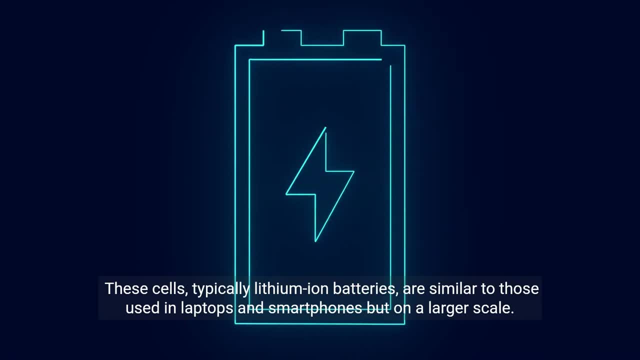 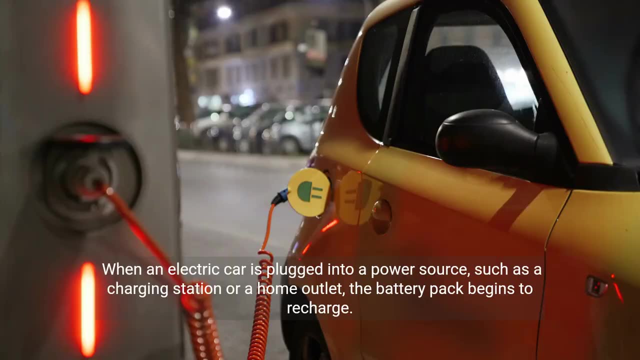 those used in laptops and smartphones, but on a larger scale. The battery pack is rechargeable and provides the energy required to drive the electric motor. When an electric car is plugged into a power source, such as a charging station or a home outlet, the battery pack begins to. 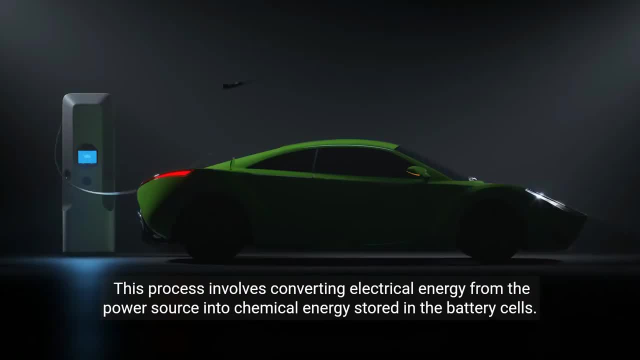 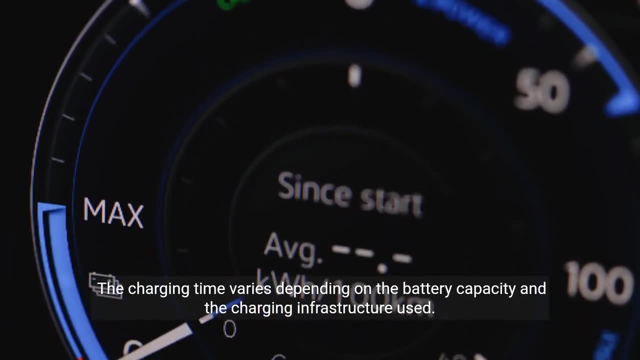 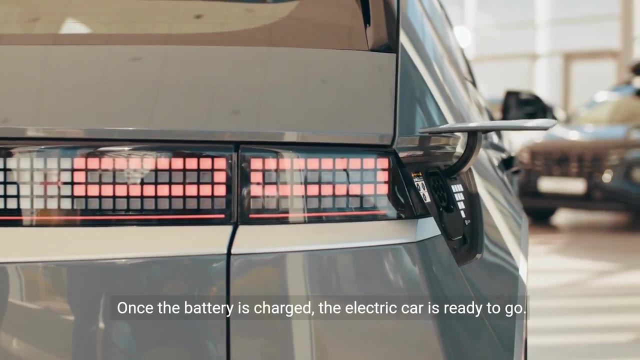 recharge. This process involves converting electrical energy from the power source into chemical energy stored in the battery cells. The charging time varies depending on the battery capacity and the charging infrastructure used. Once the battery is charged, the electric car is ready to go. When the driver activates the accelerator pedal, the electric motor receives. 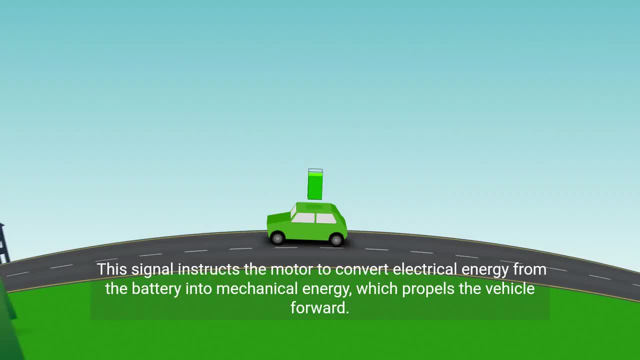 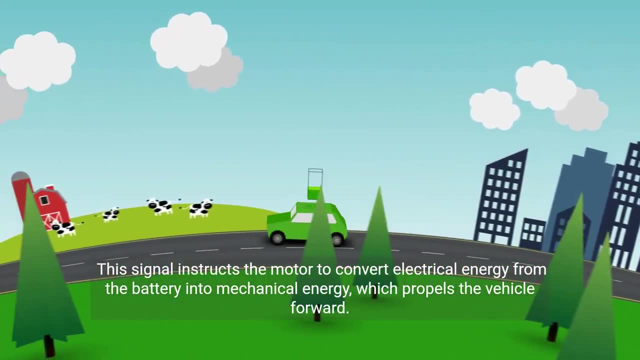 an electrical signal from the car's control system. This signal instructs the motor to convert electrical energy from the battery to the battery. When the battery is charged, the electric motor receives an electrical signal from the battery into mechanical energy, which propels the vehicle forward, Unlike internal combustion. 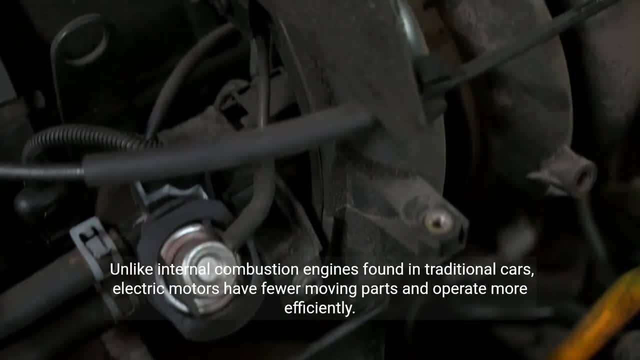 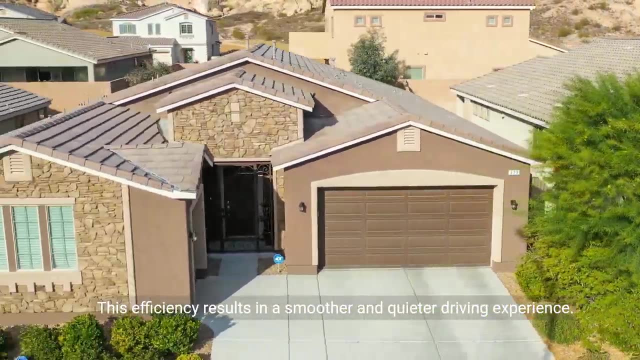 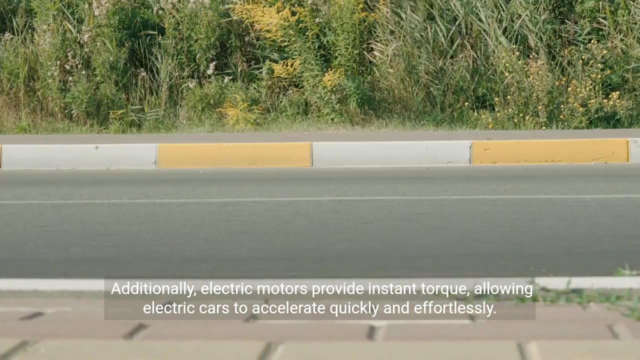 engines found in traditional cars, electric motors have fewer moving parts and operate more efficiently. This efficiency results in a smoother and quieter driving experience. Additionally, electric motors provide instant torque, allowing electric cars to accelerate quickly and effortlessly. To control the speed and direction of the vehicle, electric cars utilize a power electronics. 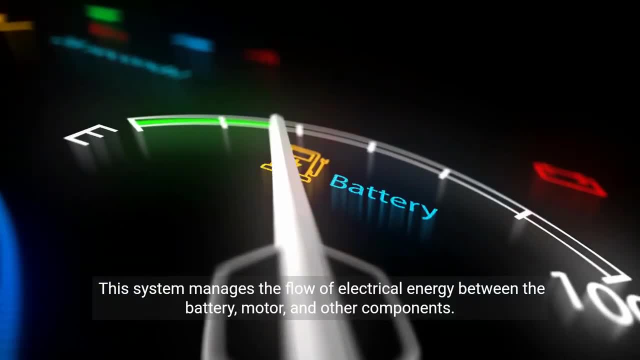 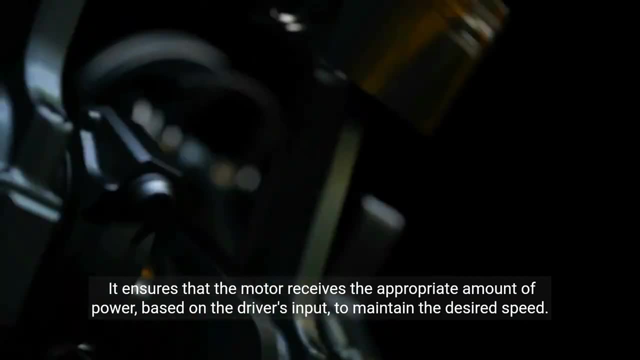 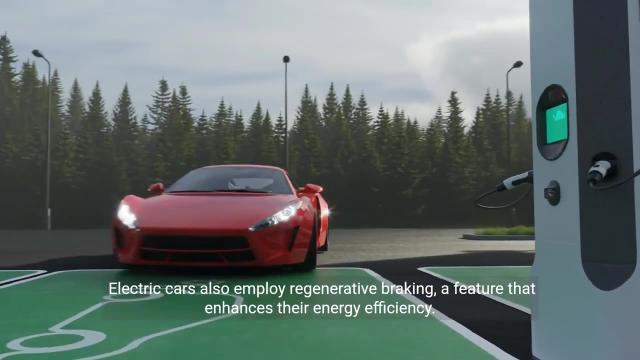 system. This system manages the flow of electrical energy between the battery, motor and other components. It ensures that the motor receives the appropriate amount of power, based on the driver's input, to maintain the desired speed. Electric cars also employ regenerative braking.